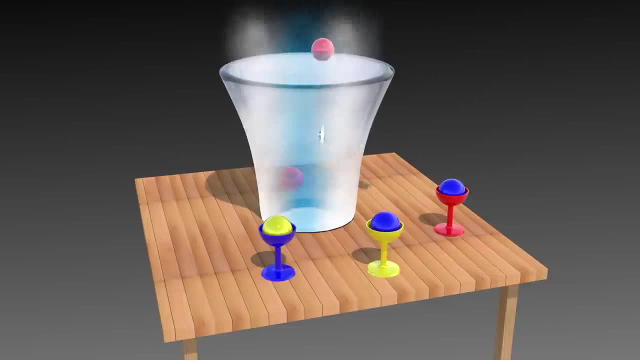 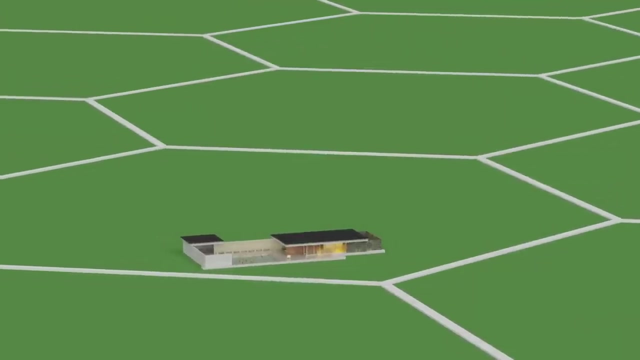 In this arrangement, there is no guarantee that this condition will be met. However, if you assign a particular size to a particular color, this condition can then be easily met. This is exactly what we do in cellular communication: The cell tower takes the place of the fountain and users take the place of the cups. 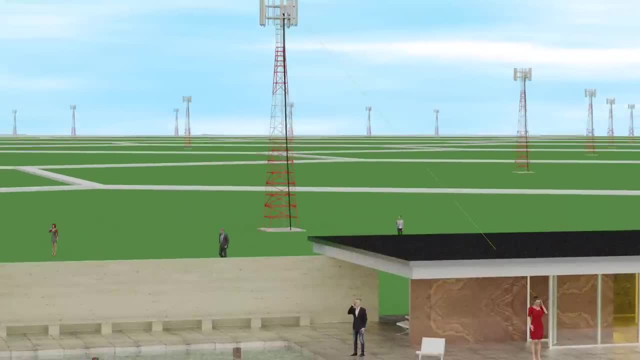 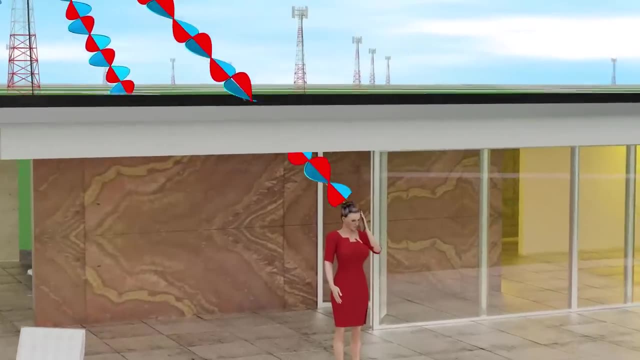 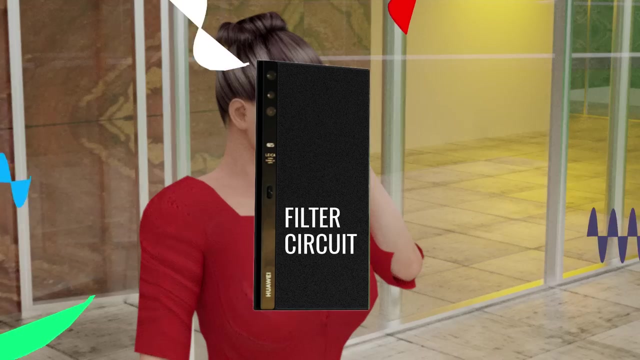 In a similar way to having balls of different sizes, we make sure that each user's frequency is unique. This way, your mobile phone will only accept the signal which has been sent, But you can also use your mobile phone to receive signals your frequency assigned to it. All other frequency signals will be rejected by your device's filter. 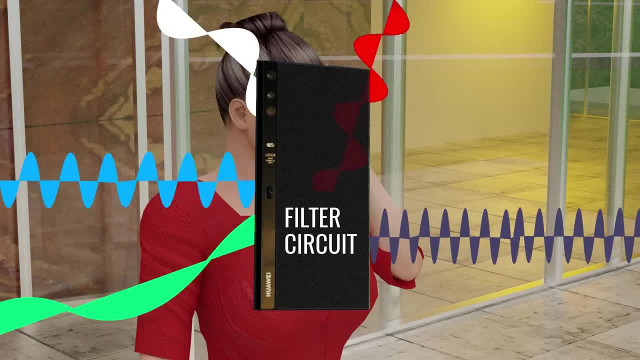 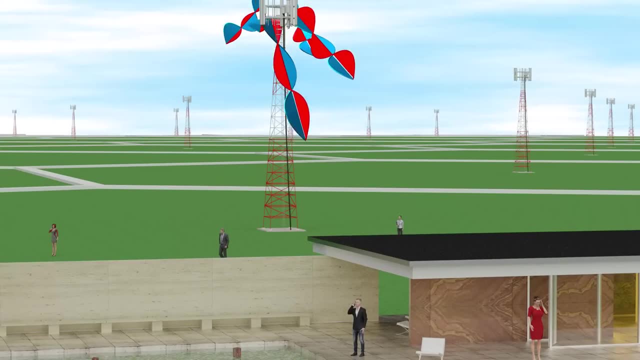 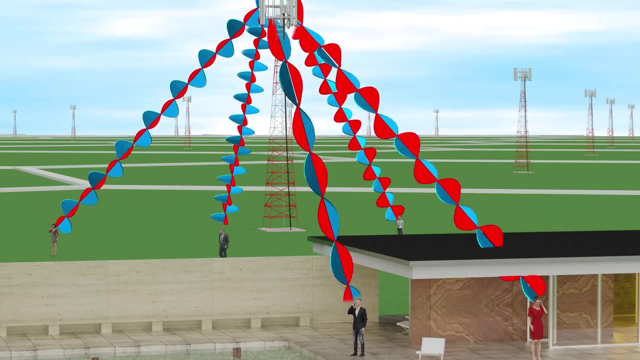 circuit. This also means each active user in the world has to have a unique frequency, otherwise you will overhear the signal of someone else. Throughout this discussion, we have kept on saying that each user has a unique frequency. However, to be precise, we should have used the. 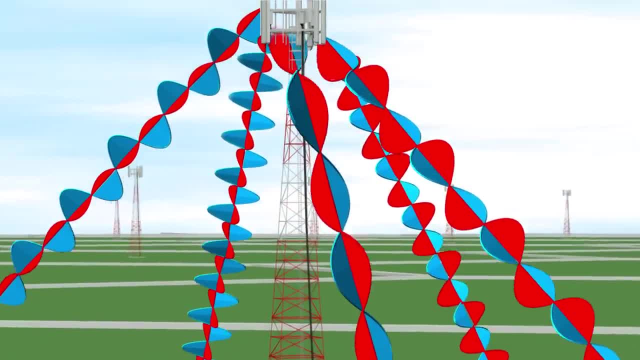 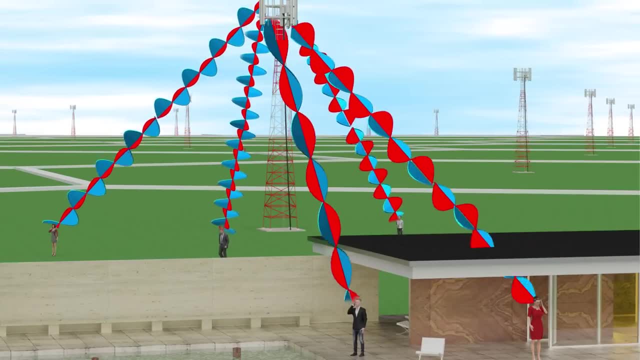 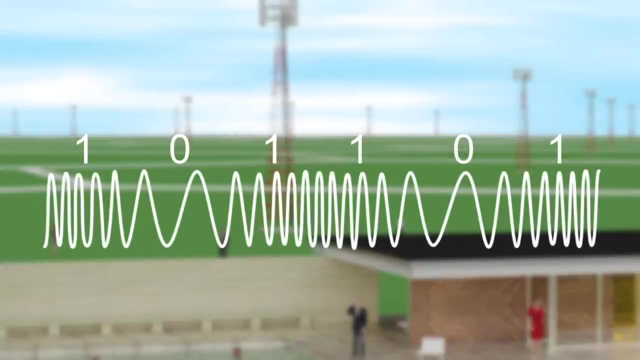 frequency range instead of frequency. Antennas are capable to transmit signals in a frequency range or band. Your phone's filtering circuit also allows a frequency band. Moreover, we need a modulation technique to transmit any signal. If we are using frequency modulation, we require two. 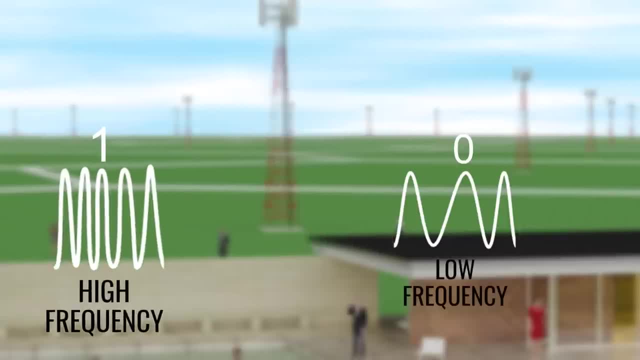 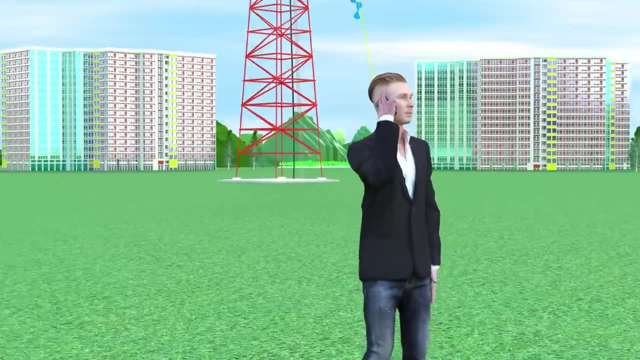 frequencies to transmit signals. The upper frequency can represent 1 and the lower frequency can represent 0.. This could lead to some questions about privacy. What happens if a hacker is able to transmit signals in a frequency range or band? If we are able to transmit signals, 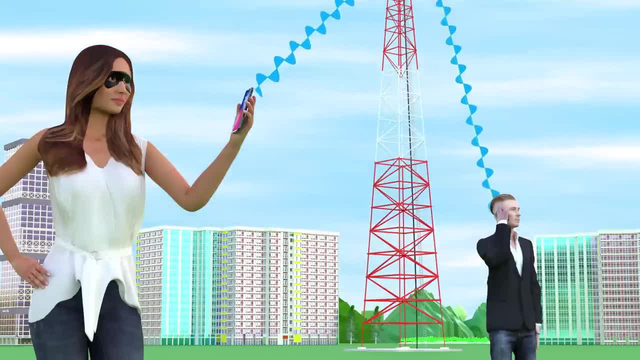 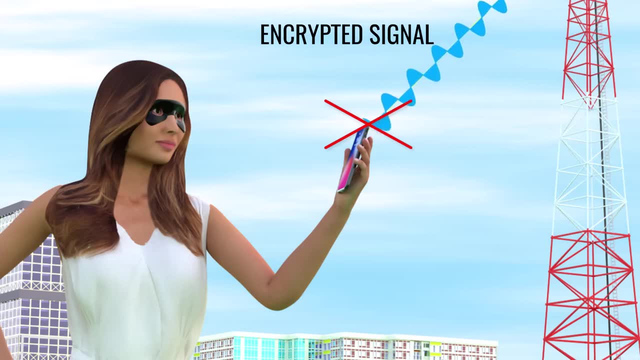 in a frequency range or band. what happens if a hacker sets our frequency in his device and tries to get access? However, it's not that simple. The signals sent over the frequency are protected using encryption, which means only your device will be able to decrypt it. In total, there are approximately. 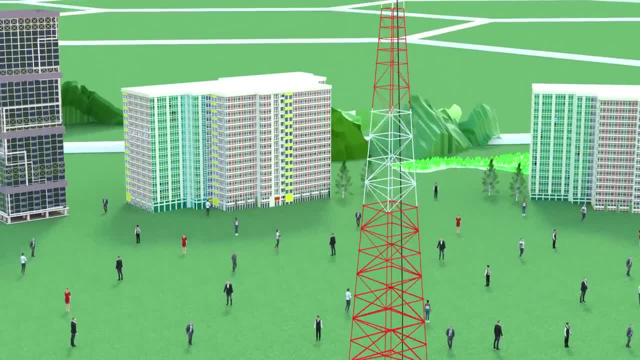 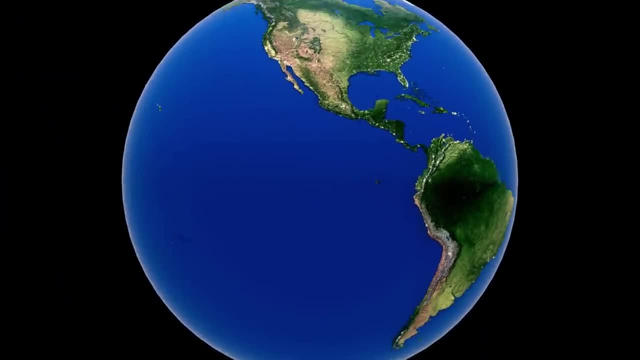 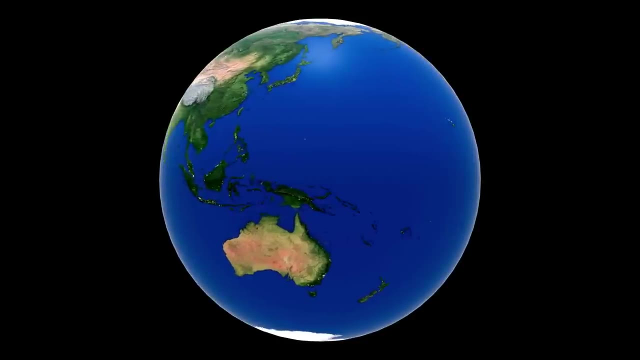 5 billion cell phone users in the world, And because the entire frequency range of the electromagnetic spectrum is not useful for cellular communications for various reasons, assigning a unique frequency range to each user is an impossible task. Let's look at the reasons why the frequency band is limited and how we are overcoming this issue. 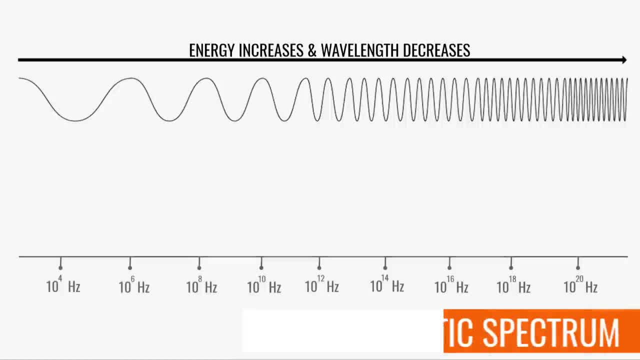 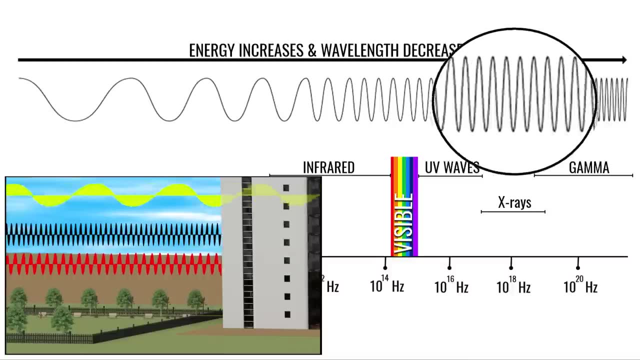 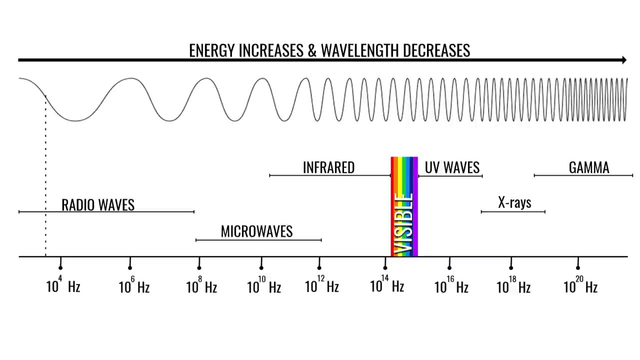 using modern technology. The electromagnetic spectrum ranges from radio waves to gamma rays. The higher frequencies of electromagnetic radiation have the worst penetration capabilities, so we don't use those frequencies for cellular communication. The lower frequencies of electromagnetic spectrum have lower energy. that would require a larger antenna for transmission. 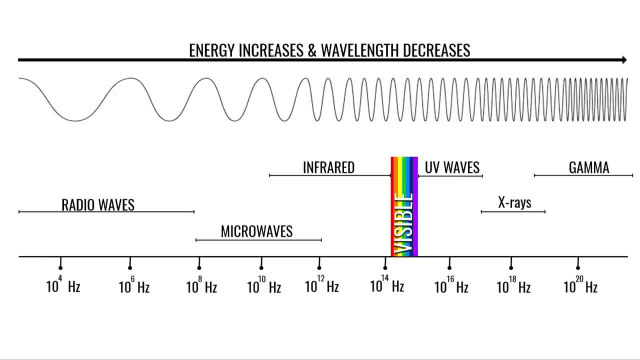 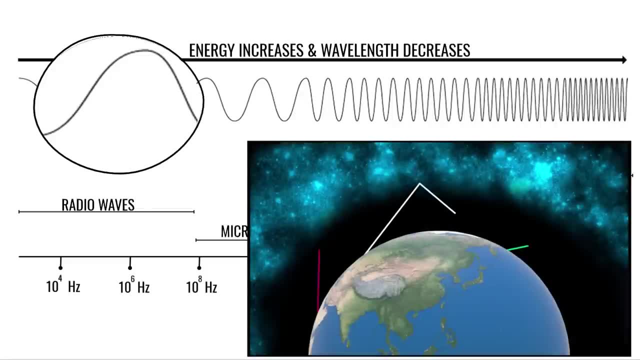 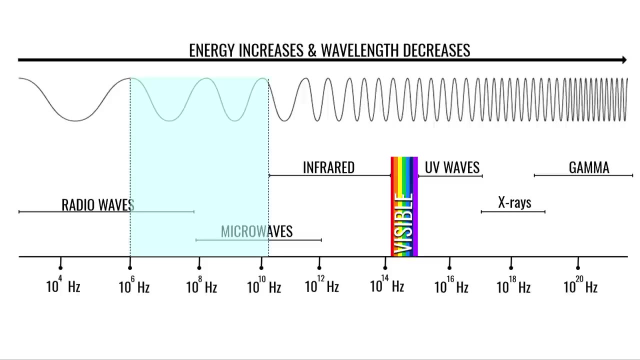 and this is practically impossible. In the next portion of the electromagnetic spectrum, as shown, the propagation is dependent on the properties of the ionosphere layer. So, due to all these restrictions, only a small portion of the electromagnetic spectrum is left. These frequency slots are also used for several 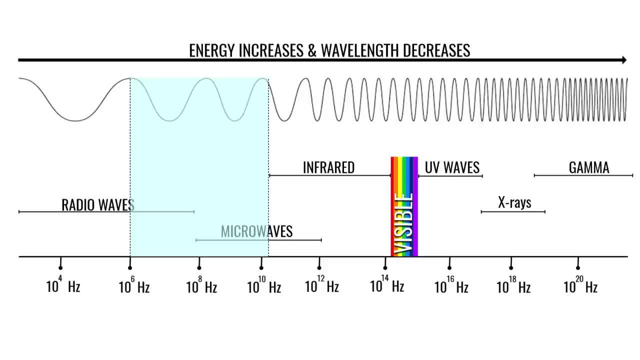 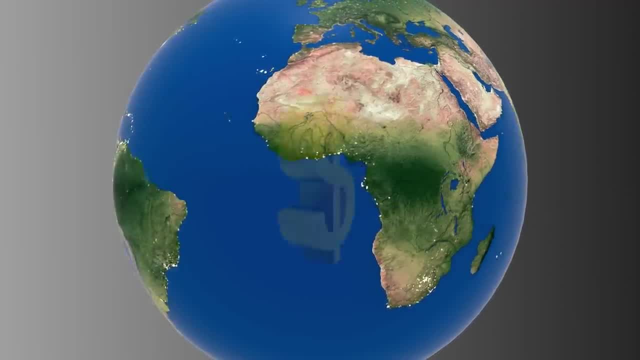 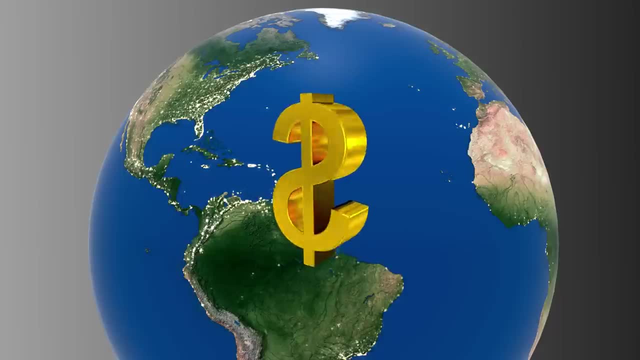 other purposes, which further reduces cellular technology's share of them. The spectrum is one of the resources which is normally managed by a government body. in most countries, The government earns by distributing various portions of the spectrum between companies using an auction or lottery system. In the United States, two agencies, the FCC and NTIA, govern the radio spectrum. 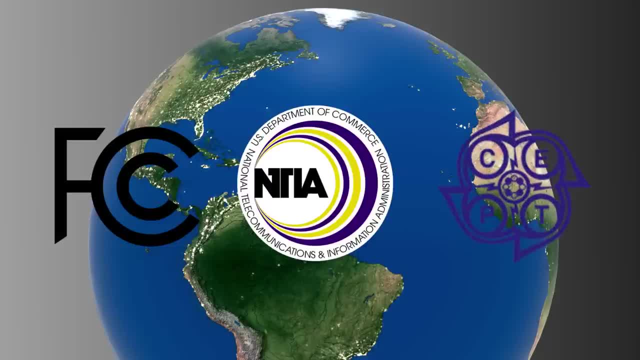 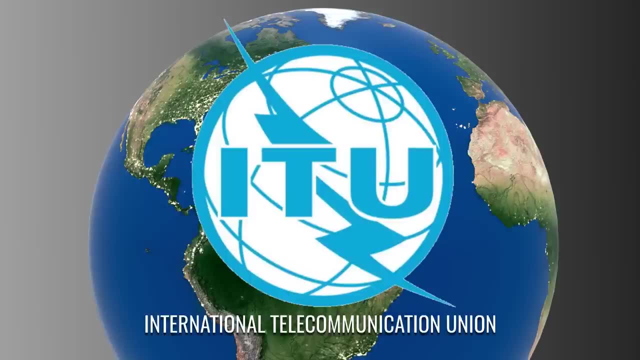 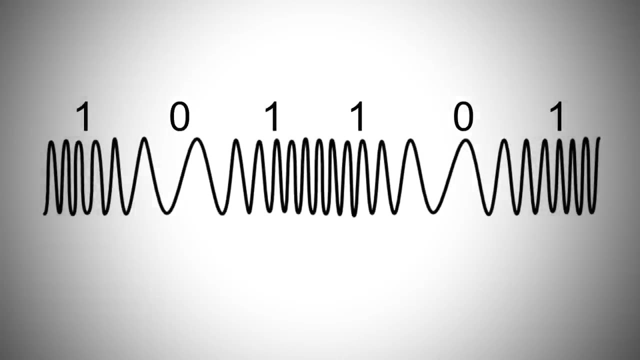 whereas in Europe the CEPT does the job At the global level, the ITU, International Telecommunication Union, manages all technical things related to this spectrum. The frequency modulation we explained at the beginning is already obsolete. It was used in 1G in analog form In the fourth generation. 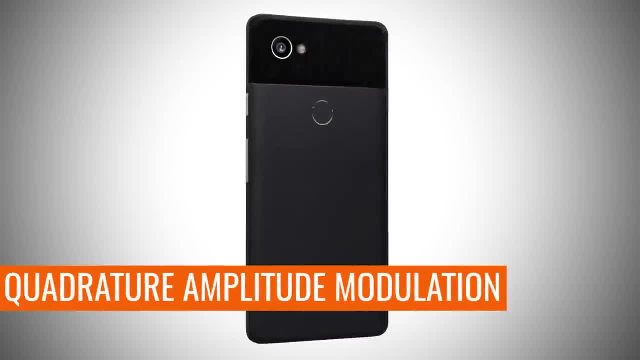 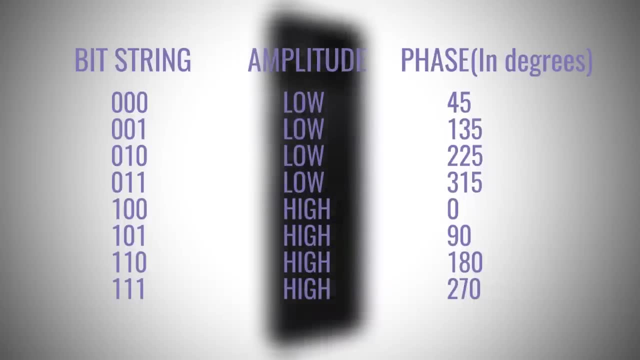 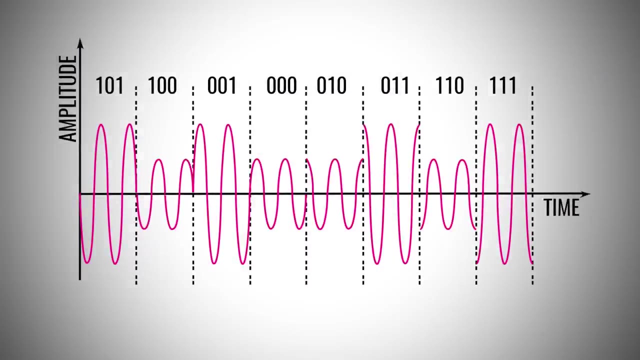 a technique called QAM is used, in which we can send more bits at a time. Let's see how it works. In QAM, variations are made to the amplitude and phasing to generate different digital signals. One such example is shown here. Hence we see that there are limited frequency ranges. 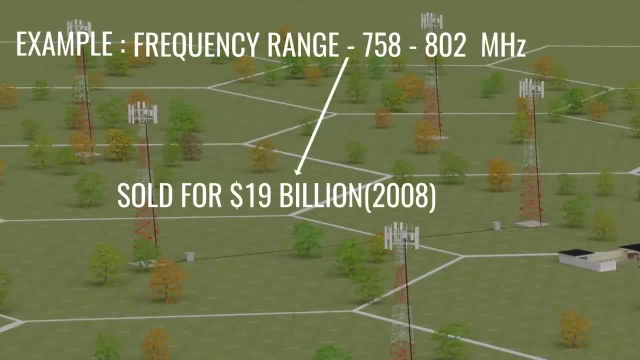 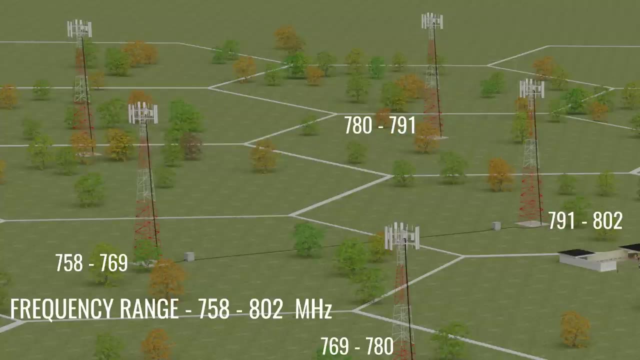 available for cellular communication, So it becomes necessary to use these ranges efficiently. To achieve this, the cellular system divides the available range into a number of frequency slots, and these frequency slots are then distributed to several towers. This distribution has the advantage of using the same frequency slot for different cell towers.